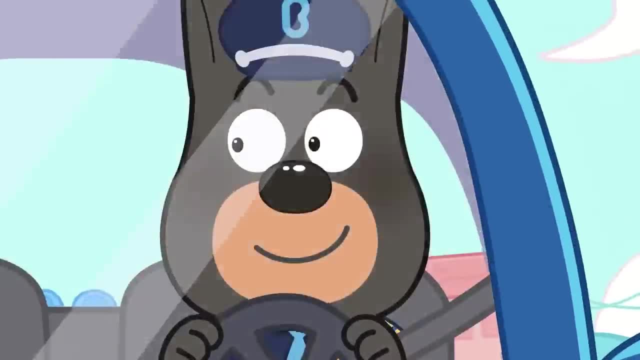 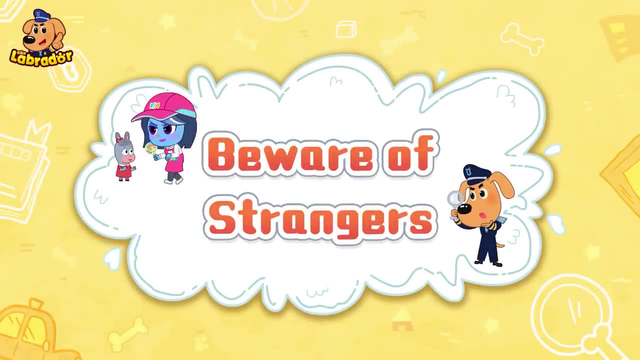 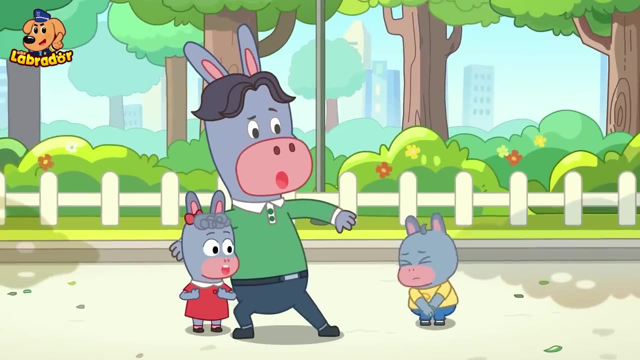 Go, Go, Go Go. Let's go, Sherry, Slap her door, Beware of strangers. Hi, Oh, Daddy, I need to go to the bathroom. Oh, there it is. Stay right here until we come back, okay. 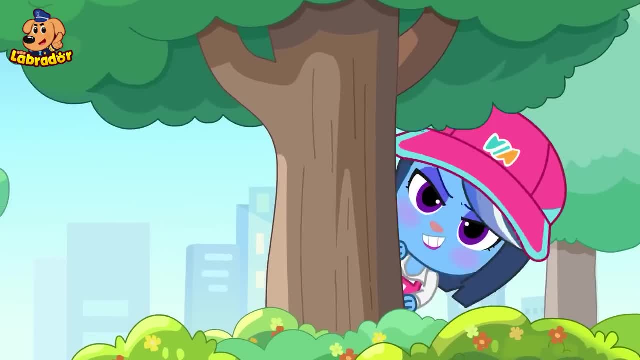 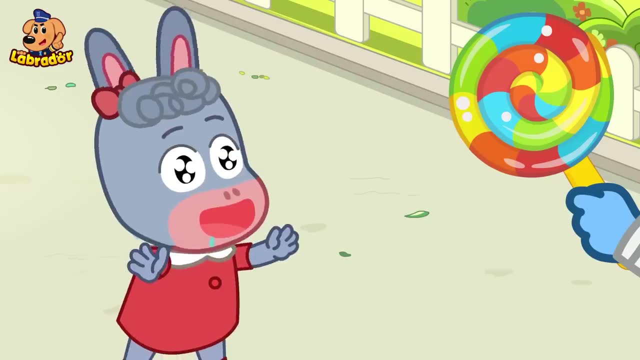 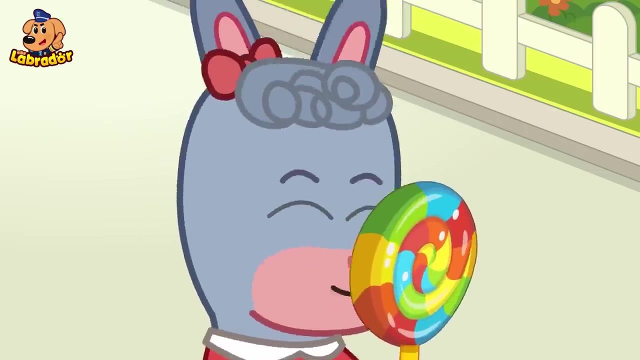 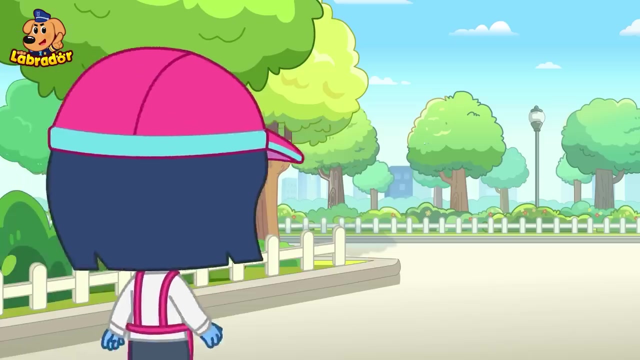 Uh-huh, Okay. Hey, kid, Do you want some candy? Wow, But… Come on, It's for you. Okay, So yummy. You can have much more in my candy shop. Come with me, But I have to wait for my daddy and little brother. 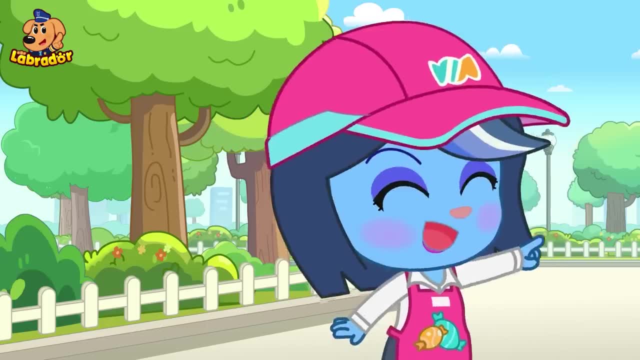 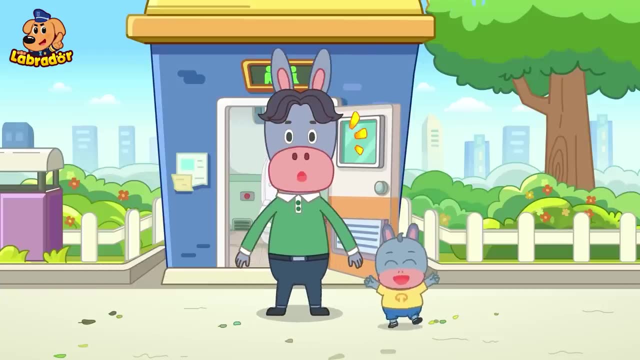 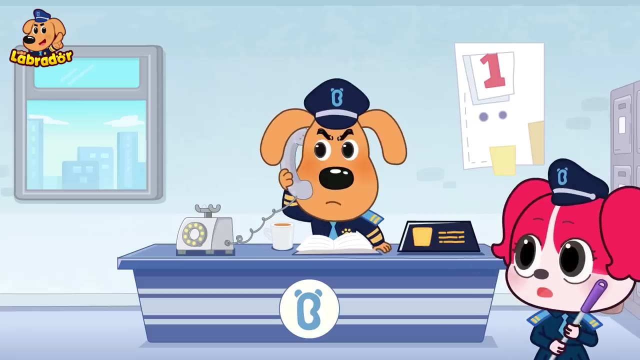 It's not far from here, It won't take long. Okay, Then I'll buy them some candy. Phew, Where did she go, My daughter? Hi, I'm Sheriff Labrador. Sheriff Labrador, My daughter is missing. Please help. 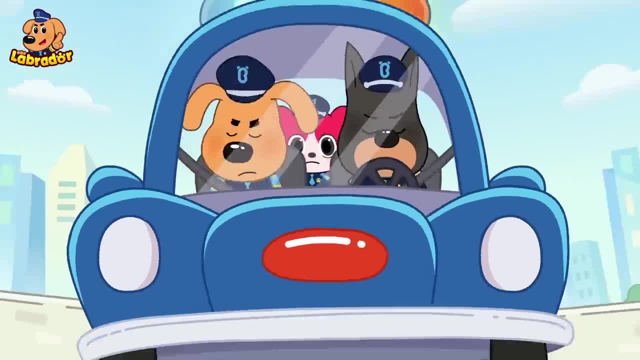 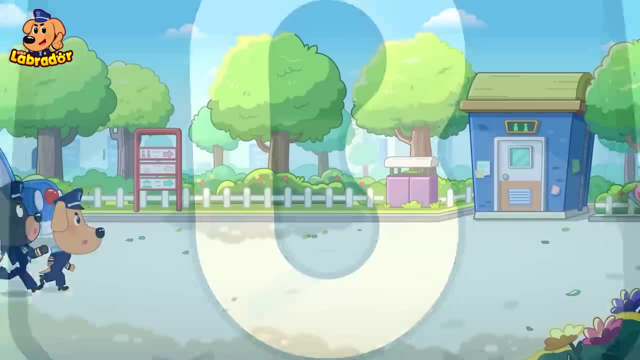 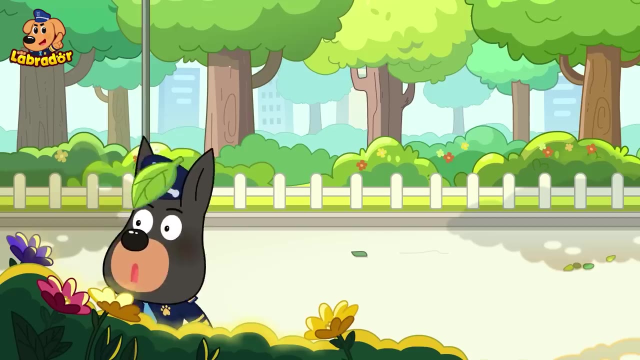 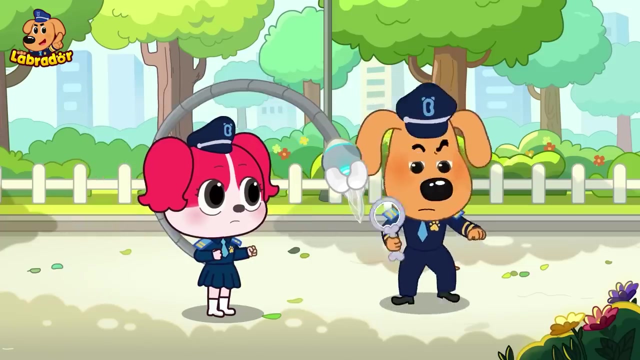 Don't worry, We'll be right there. While I was taking my son to the bathroom, my daughter disappeared. Let's split up and search. Daddy, This is a candy wrapper. These are Sister Donkey's footprints. She went that way. 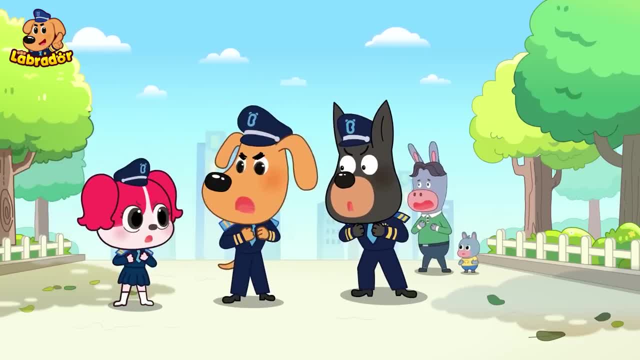 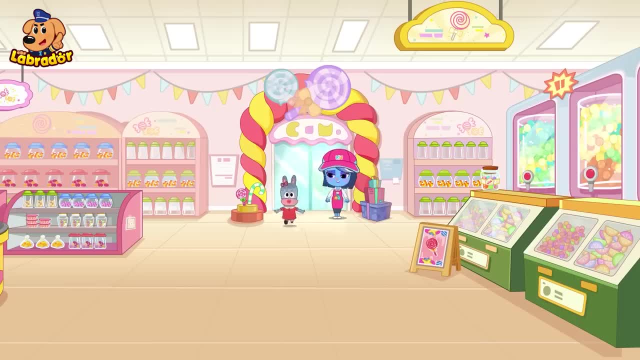 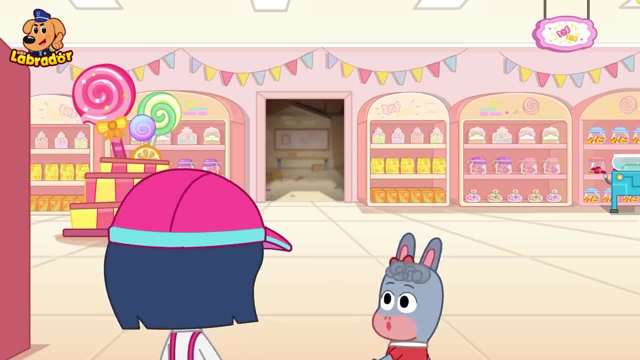 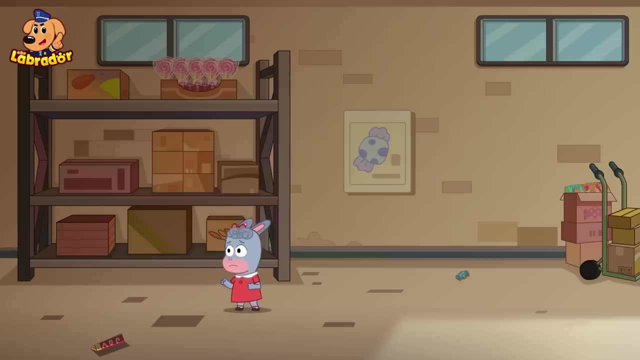 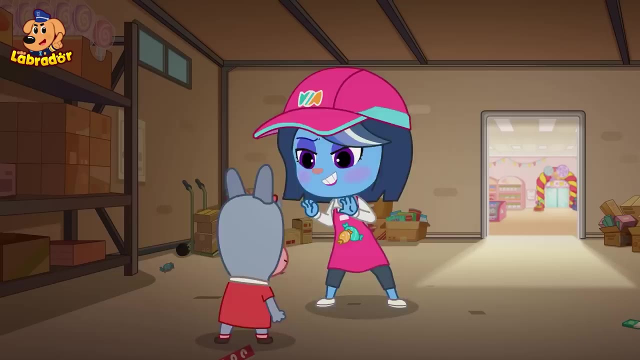 There are more yummier candies inside- Really Awesome. It's so dark in here, I'm scared. Oh yeah, Well, you can't run away, You're a bad person. Hey, Help, Help, Ouch. 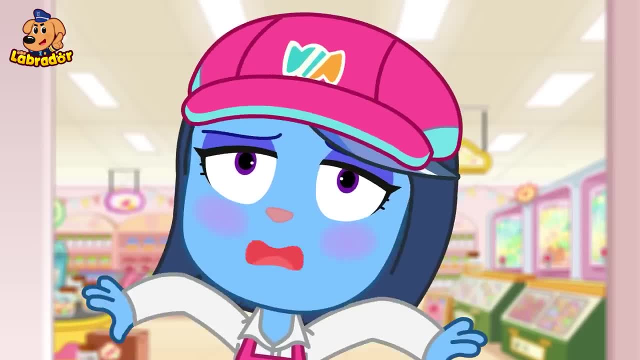 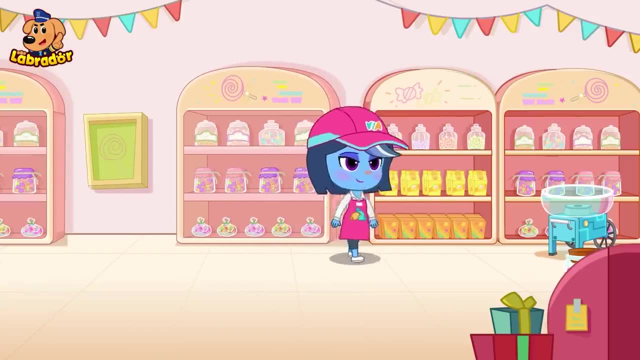 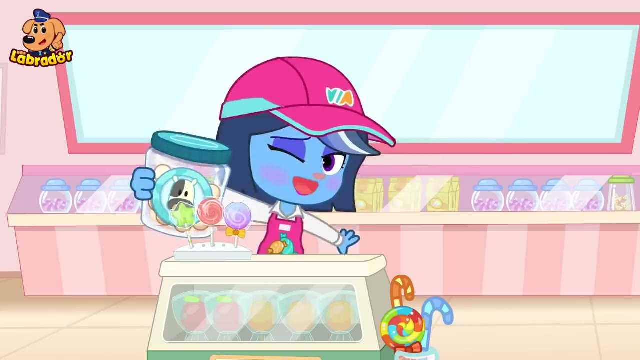 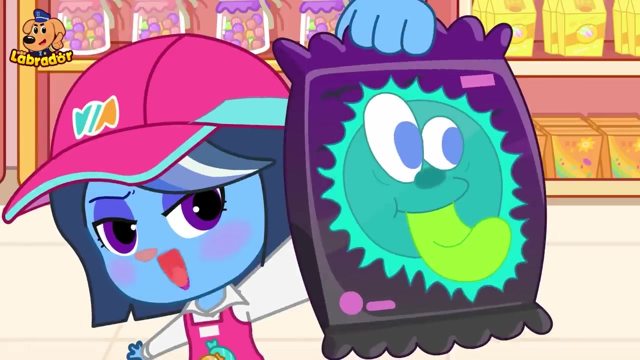 Welcome The Belize. Be quiet. Wow, Look at those candies. Welcome. What kind of candy would you like? We have fruit candy, milk candy, chocolate, lollipops, gummies And candy that changes the color of your tongue. 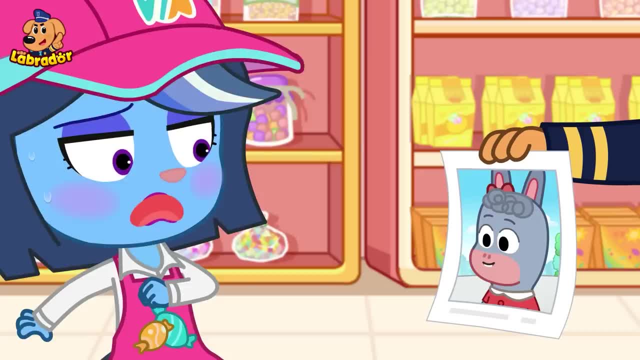 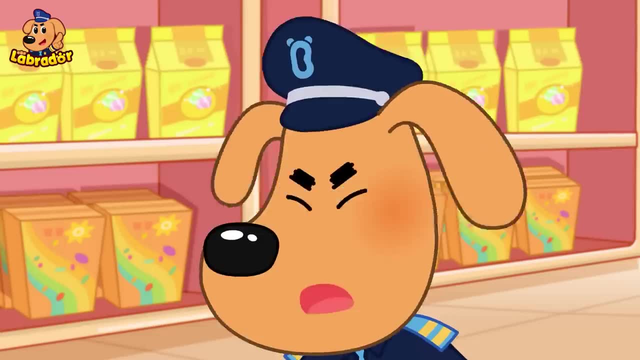 Sorry, we're here to find Sister Donkey. Oh, I haven't seen her around. You haven't? Hmm… That's right. Huh, That's Sister Donkey's hairpin, The owner's lying. Everyone look around carefully. 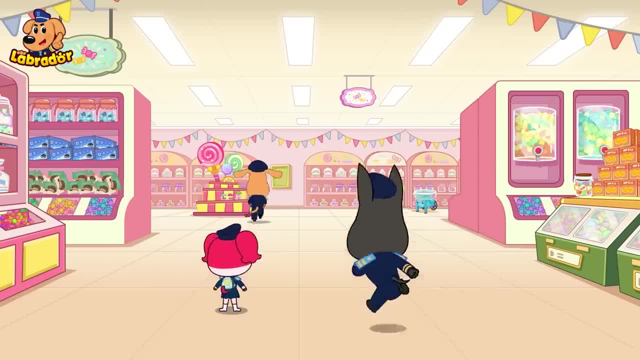 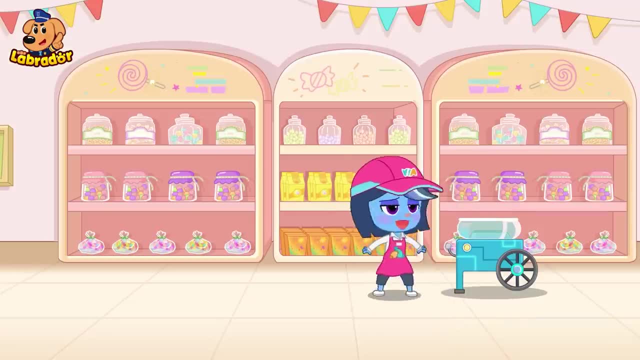 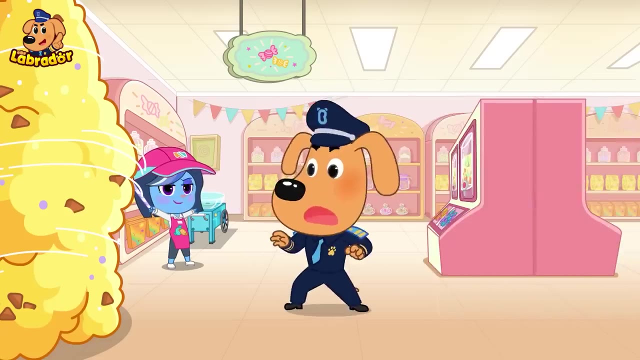 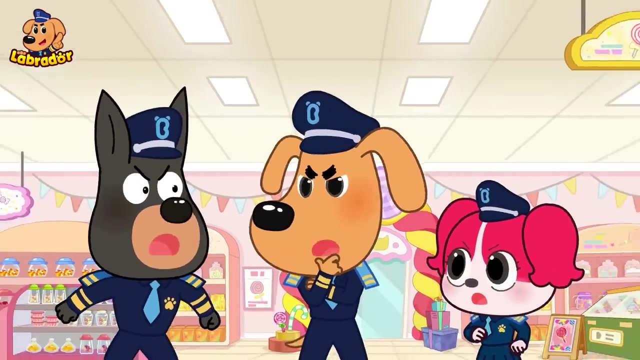 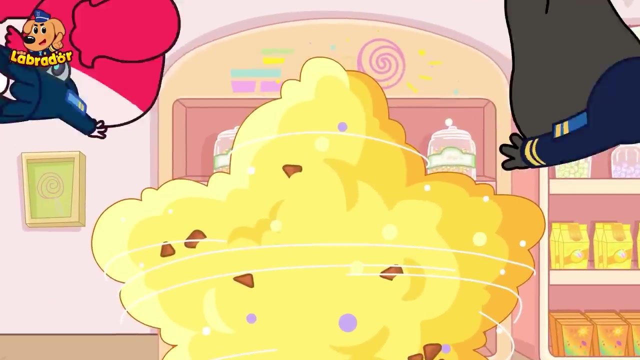 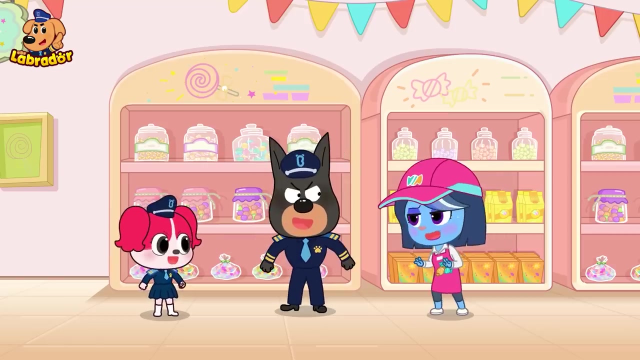 Oh no, Did they find something? Huh, This is our most popular cotton candy. It's really yummy. There must be something behind it. We know what to do. Wow, I love cotton candy Me too. Oh, What's that sound? 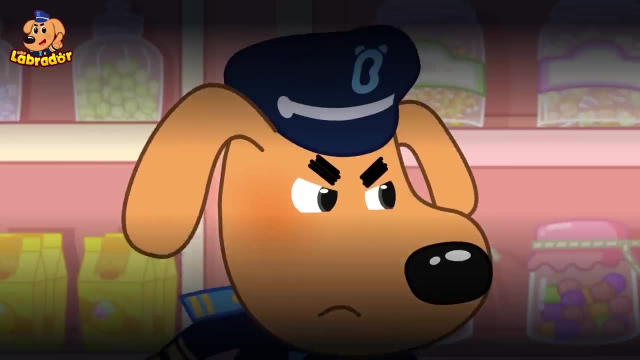 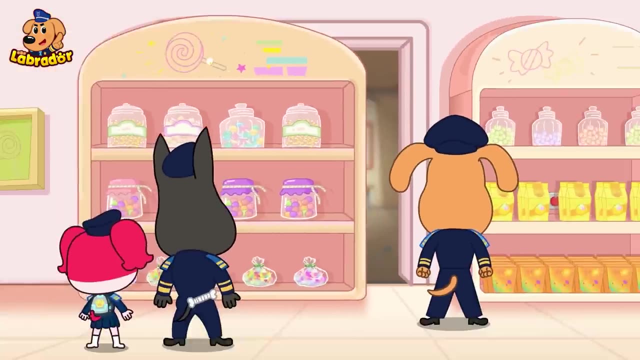 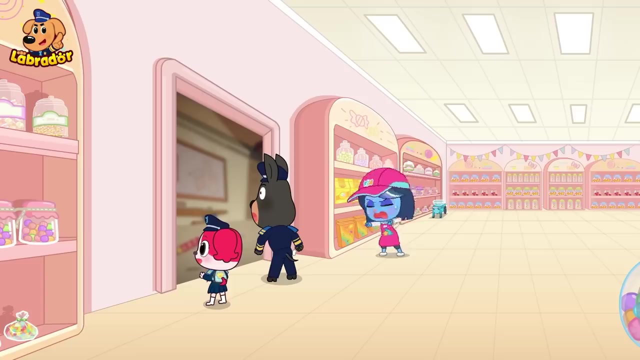 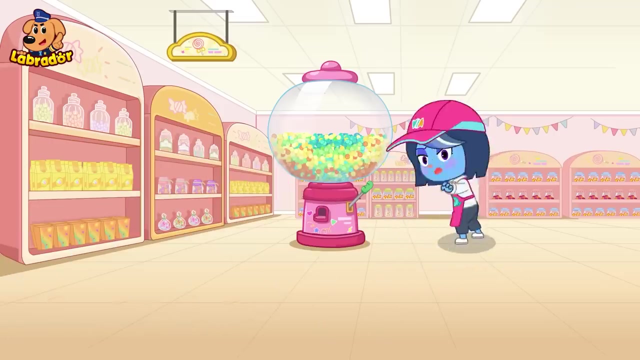 Uh no, There's nothing behind the door. Huh, Found it. There's a secret door here. Sheriff Labrador, Sister Donkey, You found her. Stop right there. I can't believe you found her. Let's see what you can do. 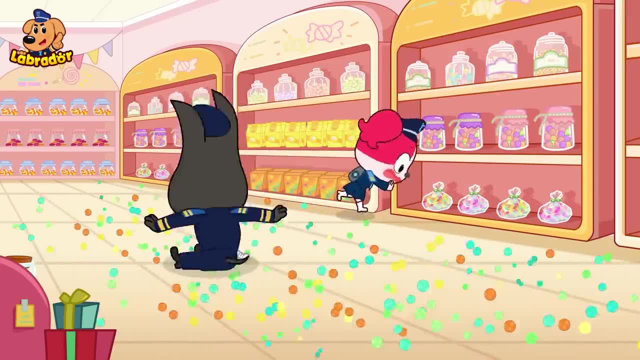 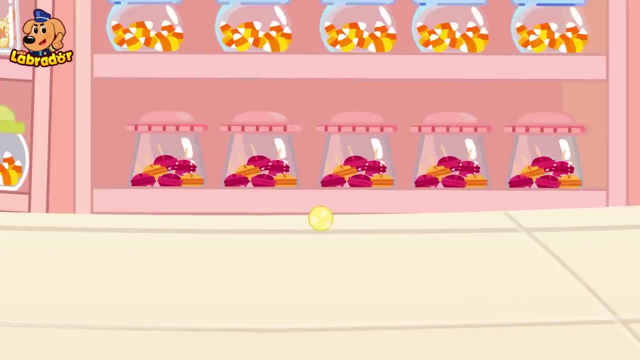 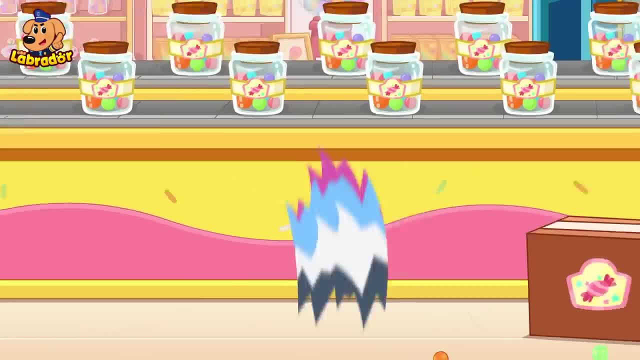 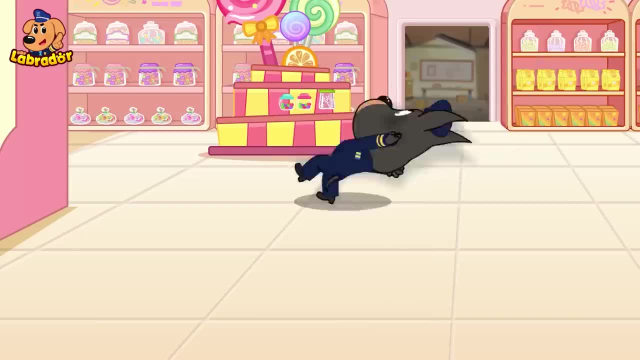 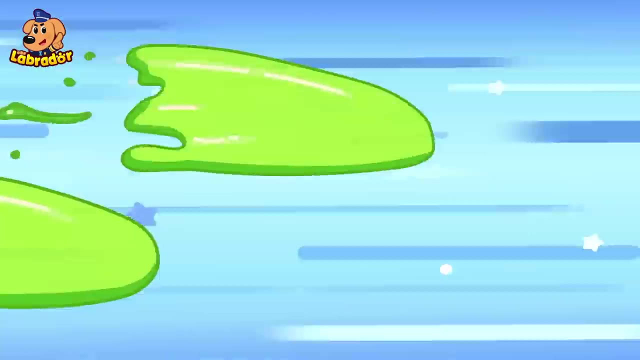